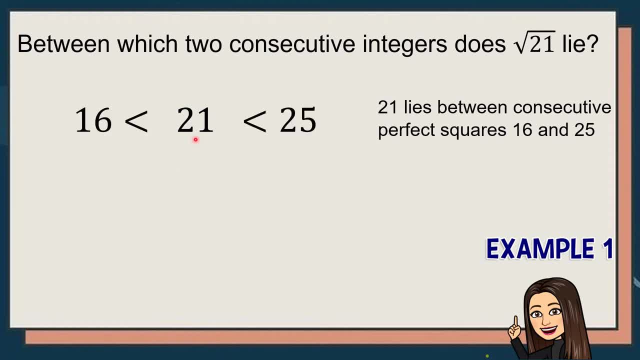 So we have here: 16 is less than 21 and 25.. 25 is greater than 25,, uh, 21.. Sorry. So again, these 16 and 25 are consecutive perfect square wherein 21 lies. Okay. Next we have to extract the principal root of the two perfect squares. 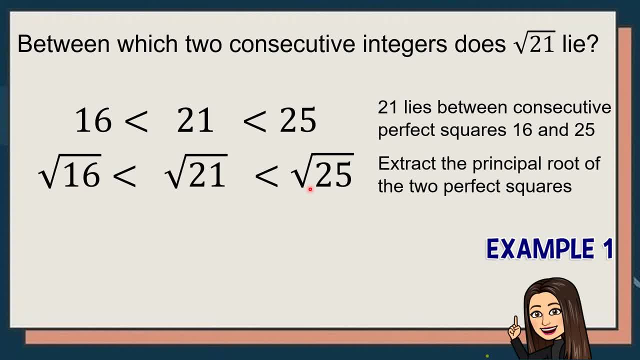 So we have to get the square root of the two perfect squares that we identified in the data box of step number one, So getting the square root of 16, so we have here 4, and the square root of 25, we have here 5.. 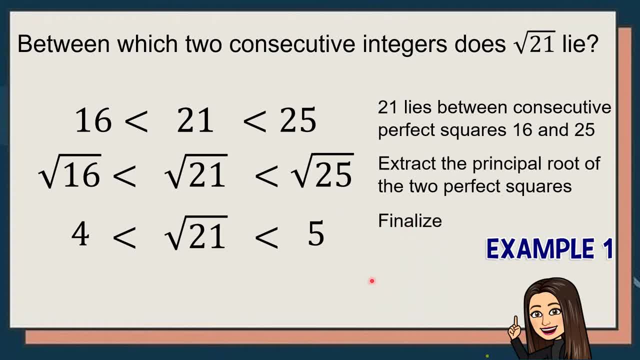 So let us now finalize our answer. So we may say that these two consecutive integers between- uh, this square root of 21 lies is between 4 and 5.. So, therefore, square root of 21 lies between 4 and 5.. 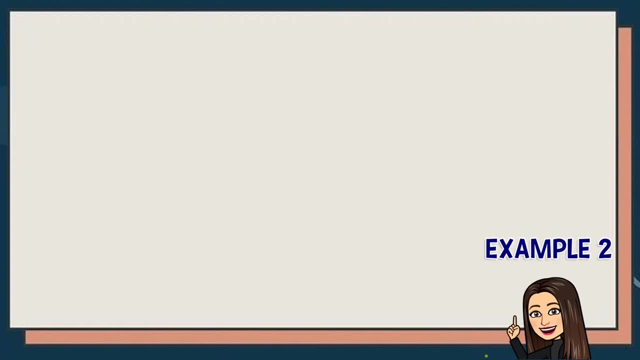 Okay. Next, this example, number 2.. Between 4 and 5. Between which two consecutive integers the square root of 89 lies. Okay, So the same procedure is what we are going to do, So we have to take out the radicand, which is 89.. 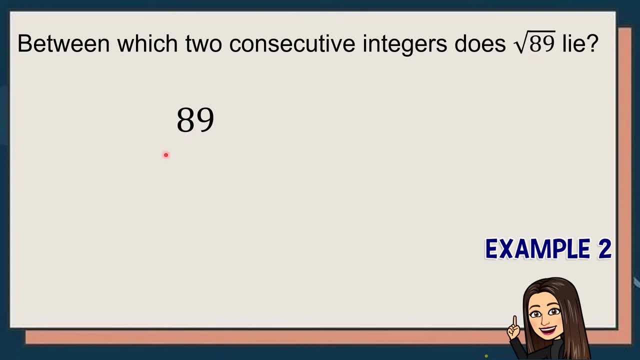 We have to think of two consecutive perfect squares that is less than 89 and also greater than 89. So consecutive, the next perfect square that is lower than 89 and higher than 89. So 89 between 2 consecutive perfect squares. 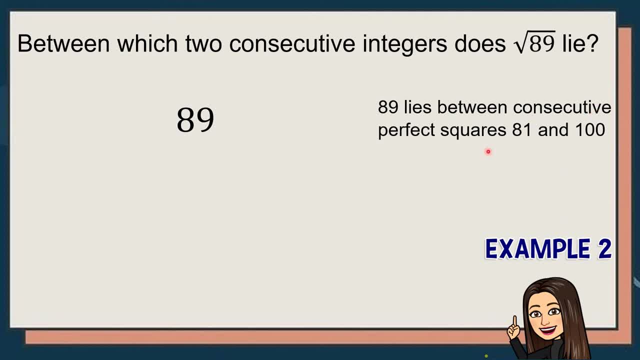 So 89 between, or 89 lies between, consecutive perfect squares which are 81 and 100.. Okay, So 89 is greater than 81, but less than 100.. So we can now proceed to the next procedure by extracting the principal root of the two perfect squares. 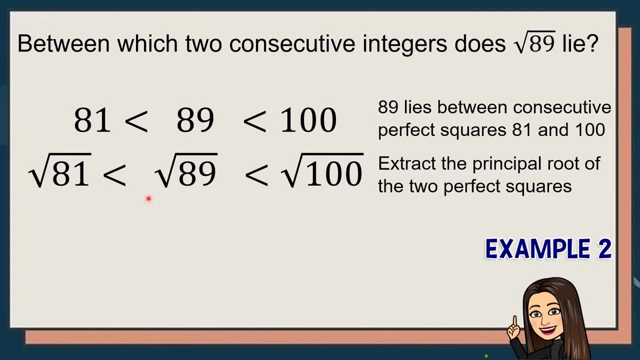 So we will get the square root of 81 and square root of 100.. So, by extracting the principal root, square root of 81 is equal to 9 and the square root of 100 is equal to 10.. So, as we finalize our final answer, we may say that the square root of 89 lies between 9 and 10..